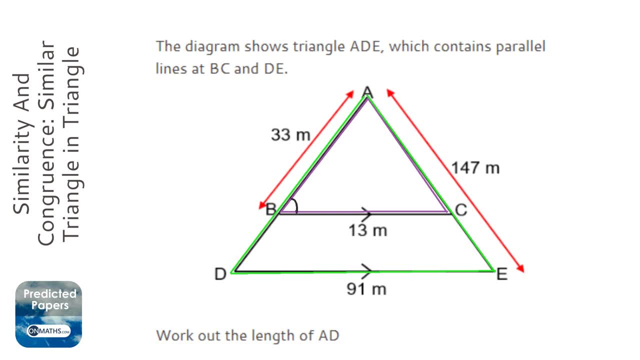 And the reason we know that is because these are parallel lines, because this angle here and this angle here will be equal. Don't need to know what they are, but they are equal because they are F angles, which is corresponding angles, and these two are also corresponding angles. 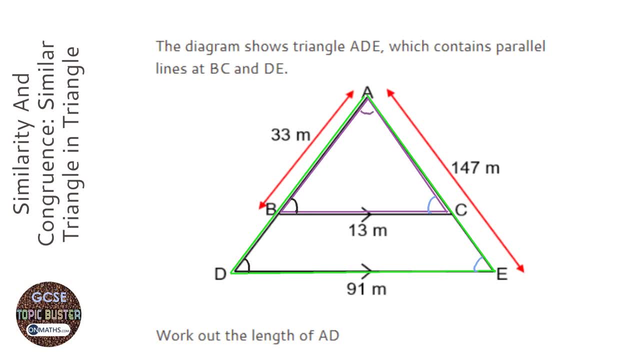 And this top one here is a shared angle between the two triangles, So the fact that they're similar, which means that we can work out a scale factor and work out missing lengths. Now the way we do this question, the simplest way of doing it. 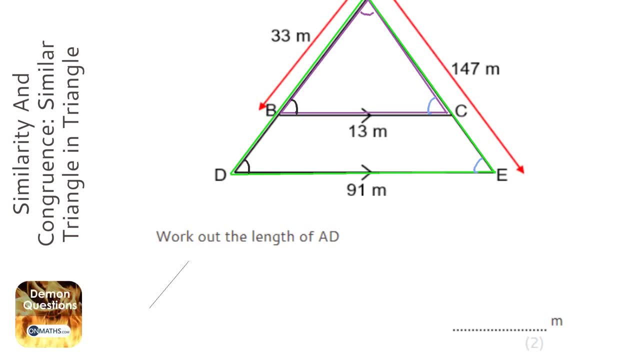 is just to draw out the two triangles. So we've got the smaller one and just do a rough sketch of it, and the bigger one and let's fill in the missing lengths. So we've got 33 here, 13 at the bottom here, 91 at the bottom here and 147 here. 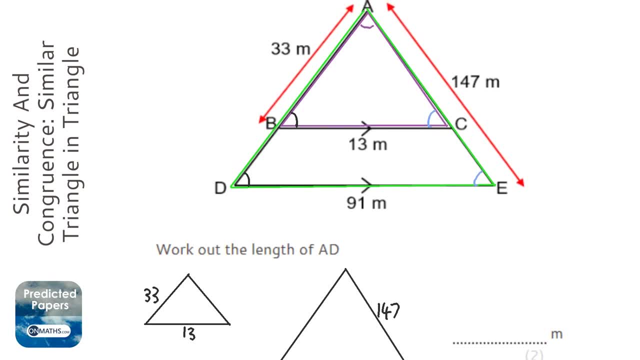 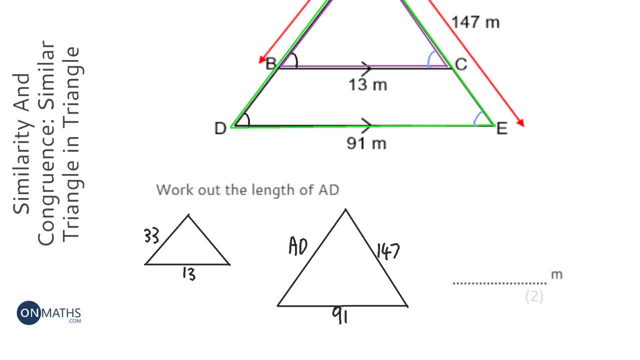 And we're asked to find length AD. Now AD is going to be this one, so length AD. Okay. so the way of doing this question will be to work out what the scale factor is. So what do we have to do to 13, to get to 91?? 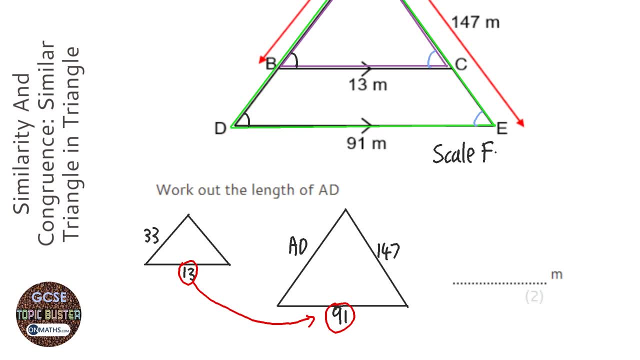 And so to work out a scale factor, we do a big length over a small length, And the two lengths need to be corresponding, which means they're the same place in both of the triangles. So we've picked the bottom ones in both the triangles. 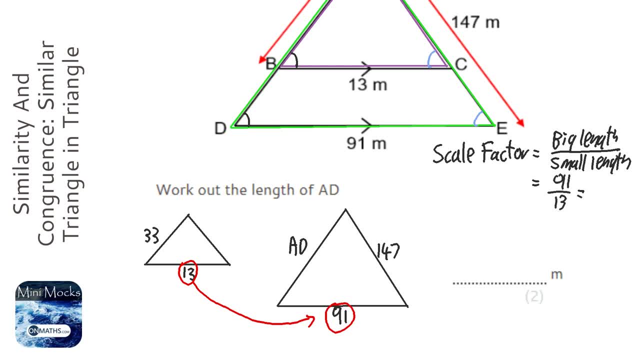 So it's 91 over 13.. And I'll get my calculator out: 91 divided by 13 is going to be 7.. There we go. So the scale factor is 7, so we times this by 7 to get here. 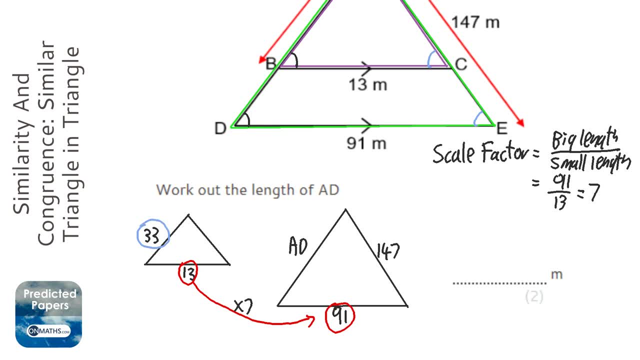 Now the problem is that we are looking for AD. So that's the question. So what do we do to that? Well, we times it by 7.. So we're going to do 33 times the scale factor, which is 7.. 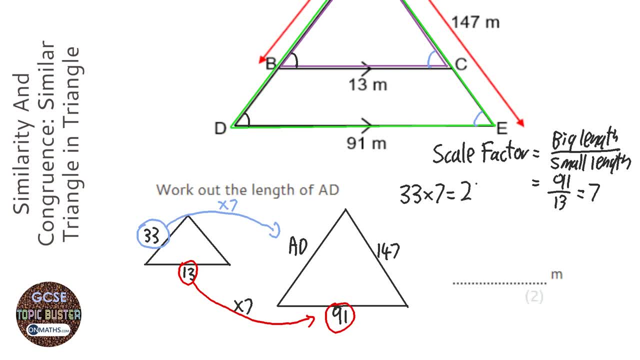 So 33 times 7, which is 231.. So it would be 231 meters. Now the last step is just to see if it makes sense. Well, it's 33 on the smaller one, so 231 on the big one.